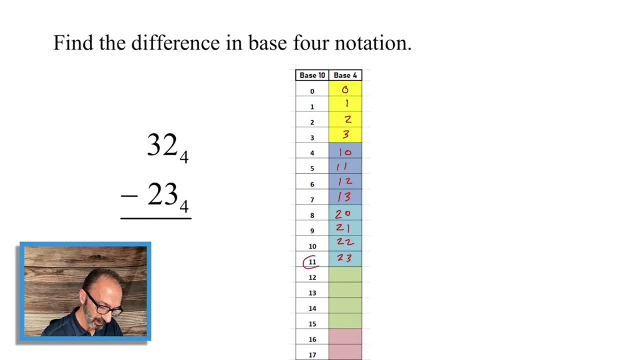 Let's look at this number 11.. What is 11? 11 in our system speaking 4s. How many 4s do we have? We have 4 and 4 equals 4 plus 4.. That's 8 plus 3. So we have 2 4s and 3 units. 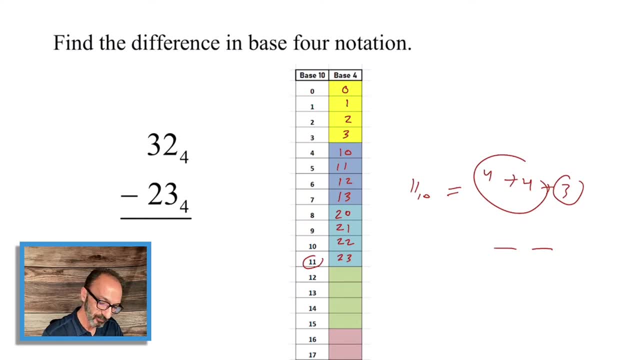 In the placeholder of how many 4s do we have, We have 2. And in the units place 3.. And that is right there, Just to let you know. To practice more. So after 2,, 3,, 3 is filled, We have to force it to be 0 and we add one more to the 2 because we can. 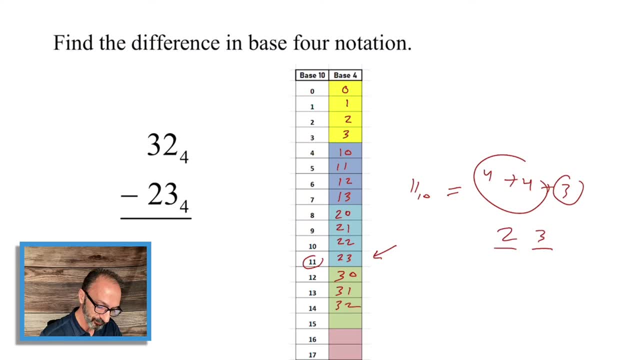 So we write 3.. Then 3, 1.. 3, 2. 3, 3.. Now both are filled. I can't add 1 and carry it to the other 3.. So what we end up with? 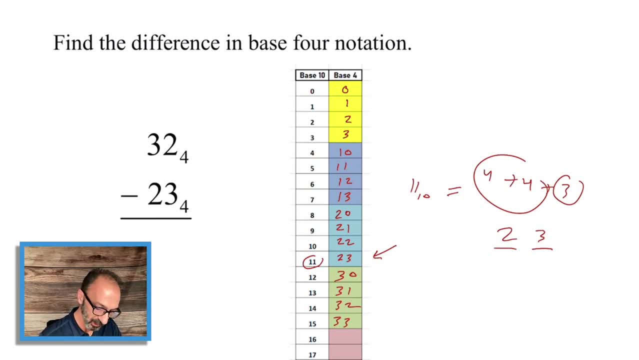 Just like in our system, 99.. After that becomes 100.. Because they are both filled, So this becomes 1, 0, 0.. 1, 0, 1.. 1, 0, 2.. And 1, 0, 3.. 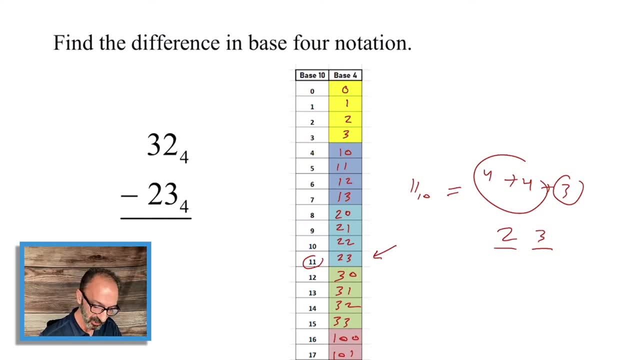 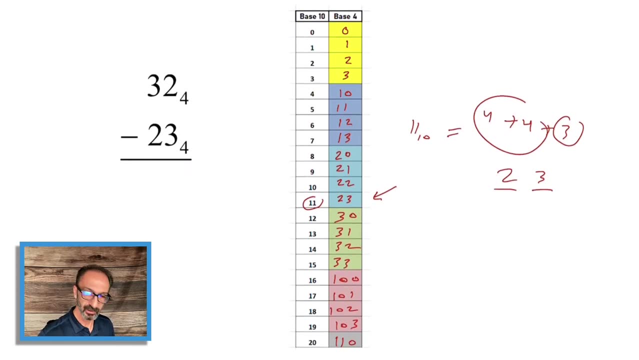 And after that 3 is filled, We force it to be 0. we add 1 to its left, Becomes 1, 1, 0.. And guess if we need more Our clear look for this, I have it. 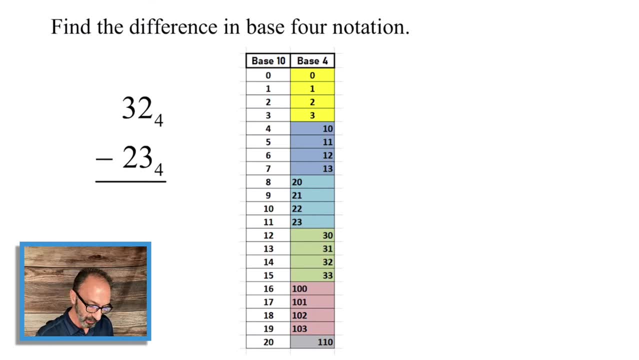 as you could see. so, uh, when i covered after 33, i think the screen was not covering that, so i'll double check with you here. when you reach to 333 or 3, 3 that means three, fours and three units. that's the meaning of it. which is 15? okay, 15 is 12 plus 3 and 12 is 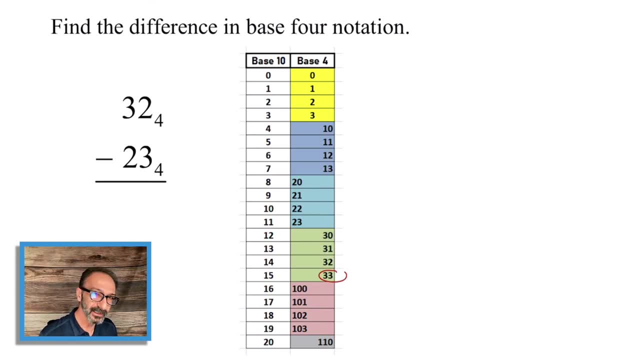 three, fourths. after that, just like 99 in our system, they're both, uh, filled. so what you do? you force them to be zero and you add one to their left. then after that, you just start filling from the right hand side and once this is filled, you need to force it to be zero and you add one to. 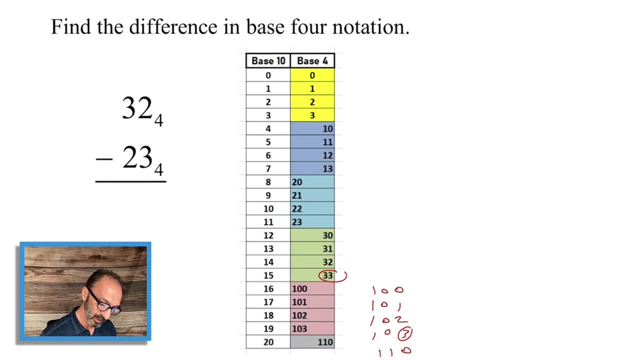 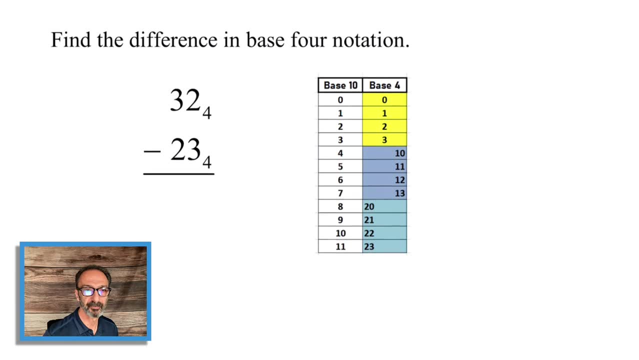 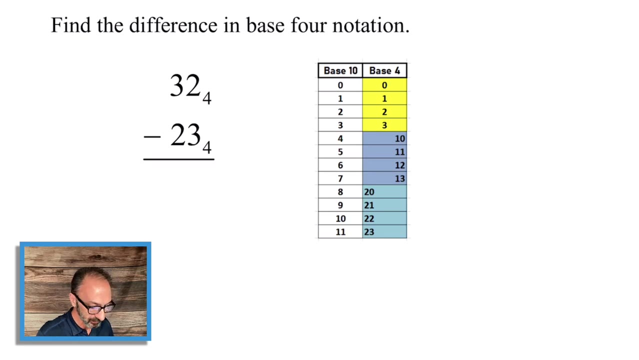 its left and you. that's why it looks like one one zero. okay, now you have it. now let's do the problem. here's the problem: we are subtracting 32 base four minus 23 base four. to do it, we're gonna go two minus three. 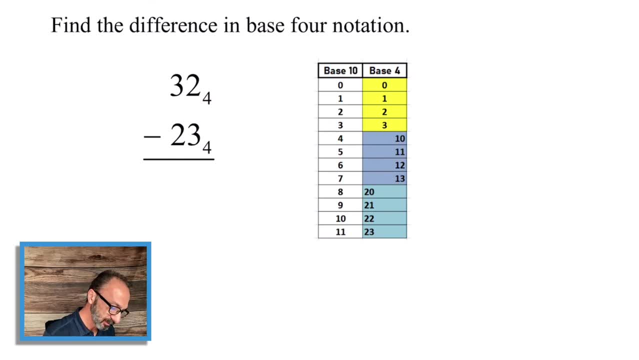 but we can't. two minus three. we can't. we need to go next and borrow one from three and force it to be two. as we do that, we go to the right and we make the two like twelve: one two, one four, because we borrowed one four from the three fours on the left. so the one two means i have one four now and two units. 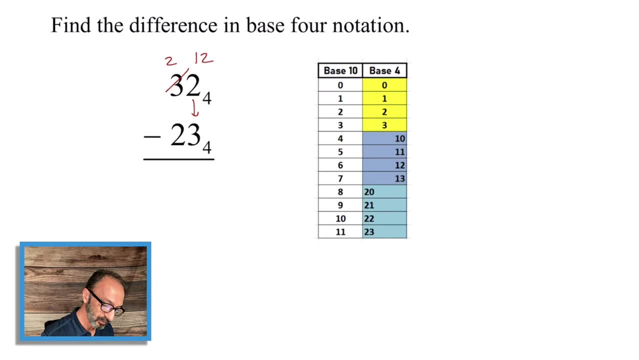 so 12 minus three. i'm saying 12. it's not 12 in our system, it's 12 in base four. here's 12 and you want to go back three. so the answer is three. so in other words, 12 base four minus three. base four should be three. 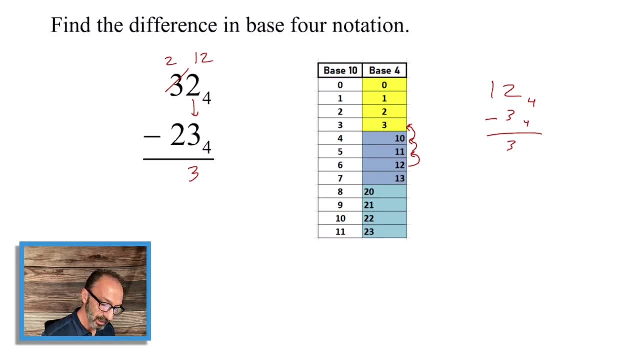 double check. you could go the other way around. you could add this to this to see if you get 12.. uh, three plus three, is it one, two? yeah, when you start here, add three more. here's one, here's two, here's three. you'll be at one, two. 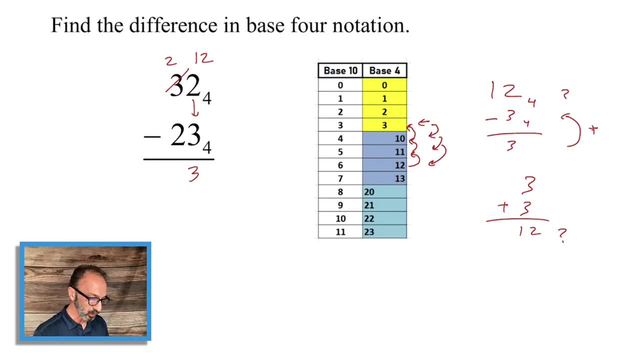 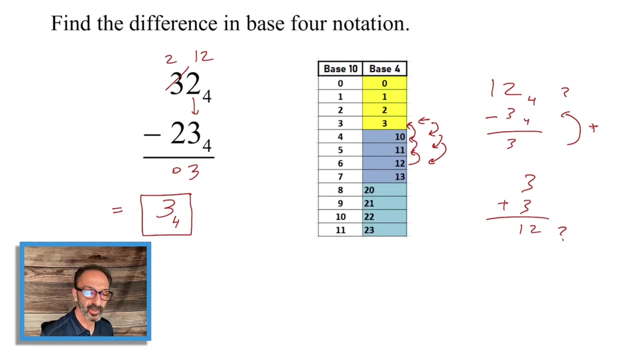 so, just like in our system, it does work. so now we come to the second column, two minus two, which is zero, and we're done. so what's the answer? the answer is three base four, and that is our answer. okay, let's double check again. we could do that by saying, okay, i'm gonna take three. 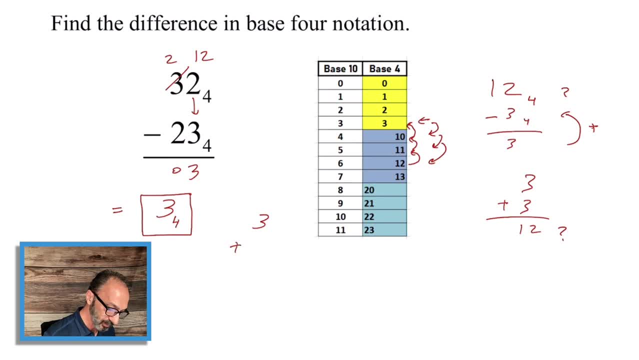 which is my answer. add it backwards and see if that's gonna give me three, two, add it to two, three and let's see: three and three is six, but six in base four is one, four and two units. one, four and two units. we carry the one and we are the two units. one and two is three. so